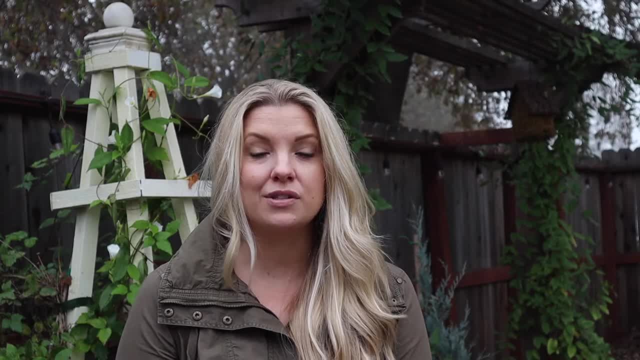 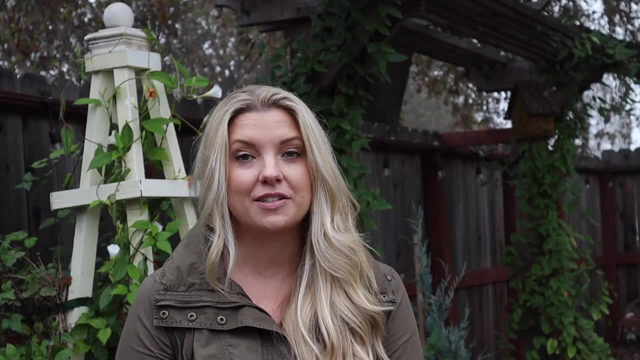 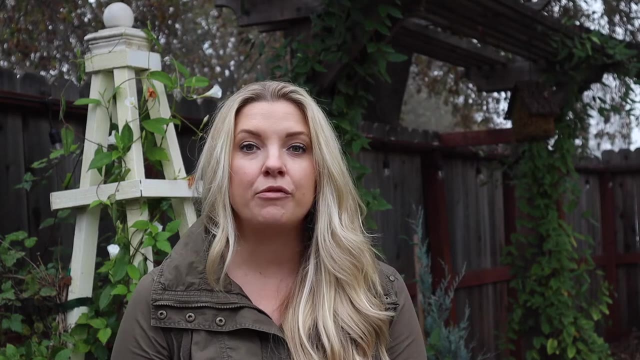 everything I know from trial and error, YouTube videos, blogs and library books. When starting this gardening channel for YouTube, my aim was to inspire small home gardeners to start their gardening journey, and I think the most important thing is to start with the basics. I remember two. 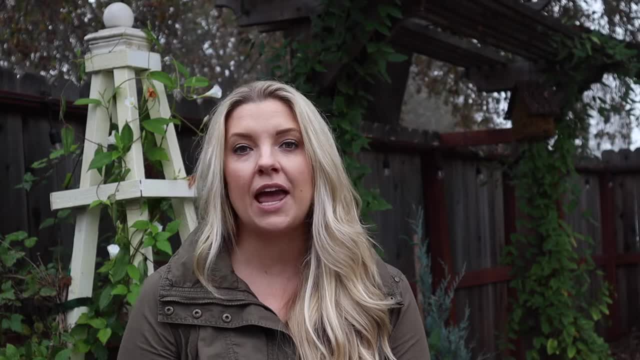 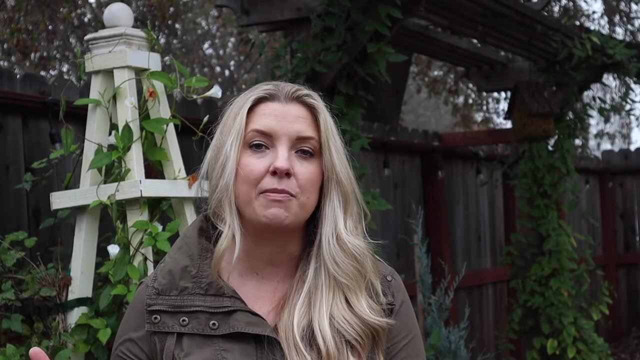 years ago, when I was starting my gardening journey, not having any idea what was being talked about in gardening videos and in books, and I had to look up every vocabulary term before I knew it- I knew what I was actually supposed to do in my garden, So I'm really excited about the video. 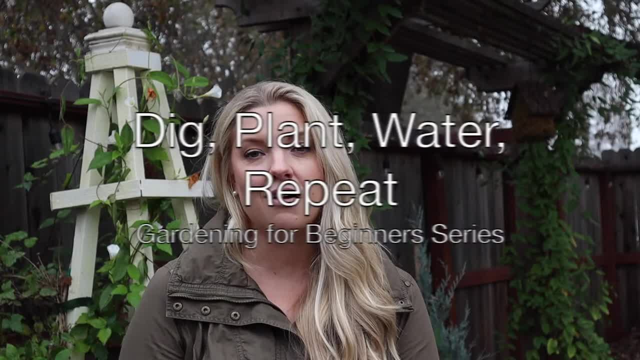 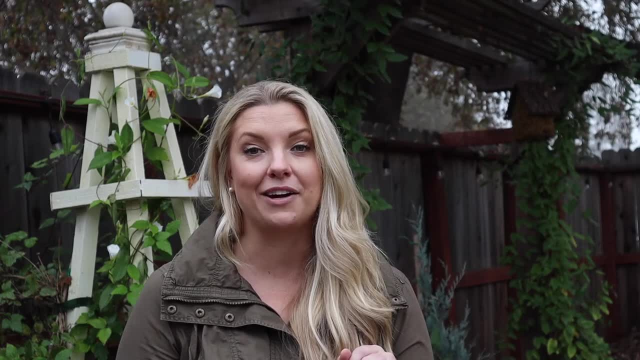 today. Today is the first video in my gardening for beginners series. I plan to get into the nitty-gritty and the basics of gardening for all you new gardeners out there. I plan to release a new video every Monday on my channel, So if this sounds like something that might be interesting, 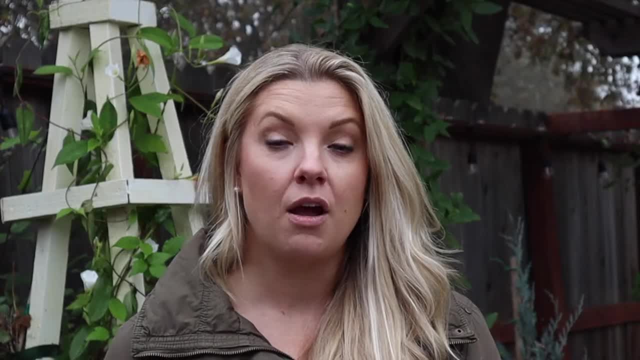 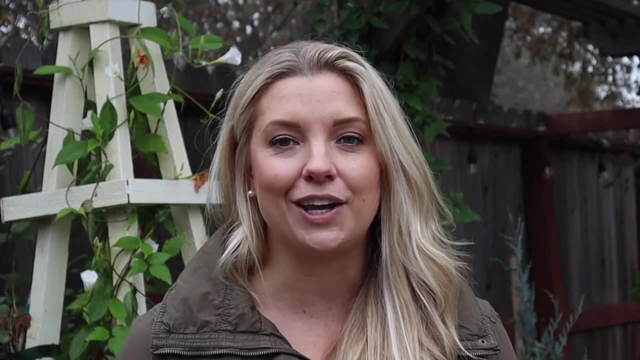 to you. please subscribe. Every week we'll work together, working through the essentials and the gardening season. If you're interested in learning more about gardening and how your garden is in full swing, you guys will be ready to go. Now let's get into the gardening basics for beginners, starting with eight easy steps. 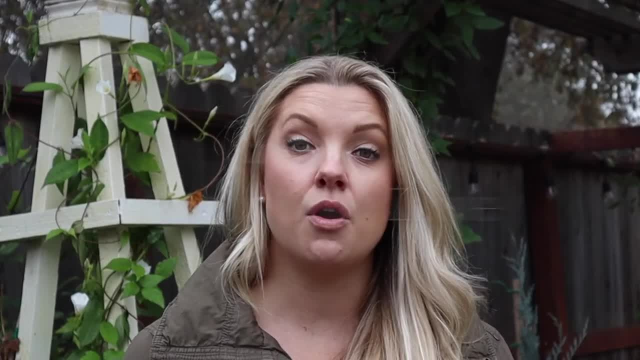 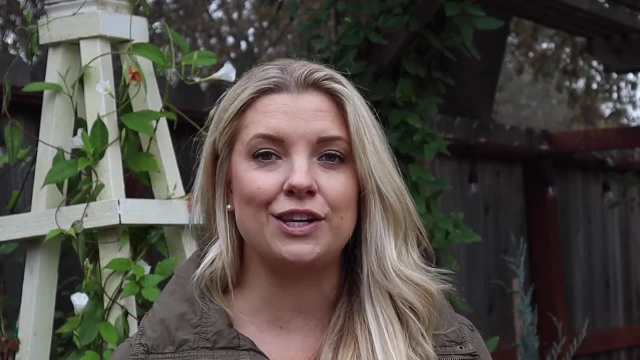 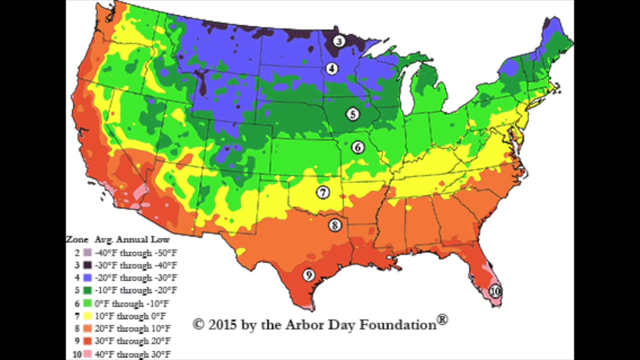 Okay, now let's start with step one, which is know your zone, and this is really important if you watch videos or read books that are written by gardeners that live in different climates than you and thus different zones than you. The map is divided up into USDA hardiness zones, which defines a certain 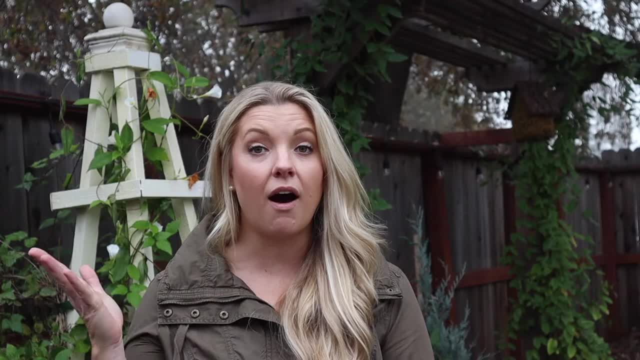 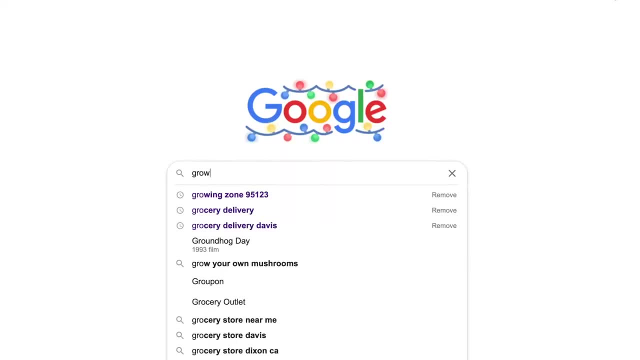 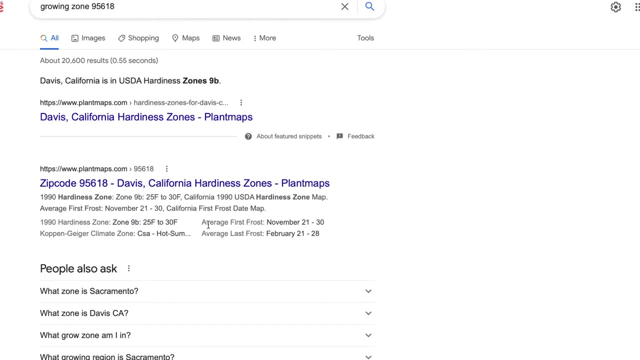 range of climate conditions. This will tell you how hot and how humid your garden is and how hot your garden is. This will tell you how hot and how cold your area is, and thus what plants will survive and thrive in your garden. To find your zone is very easy. Just type into Google something like growing zone and then your zip code and your zone should pop up right away. 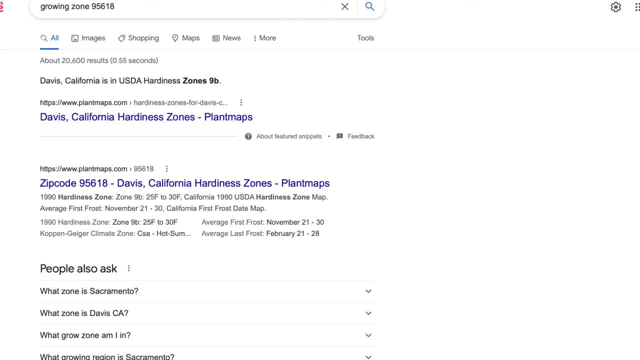 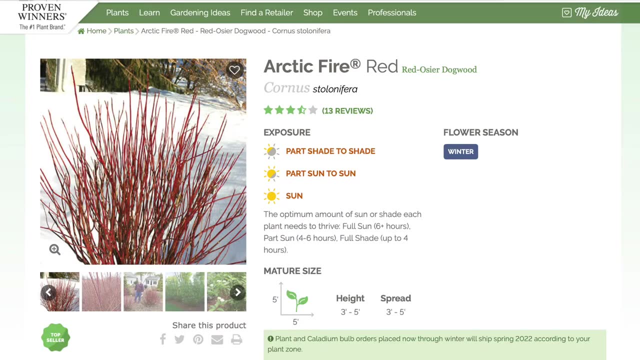 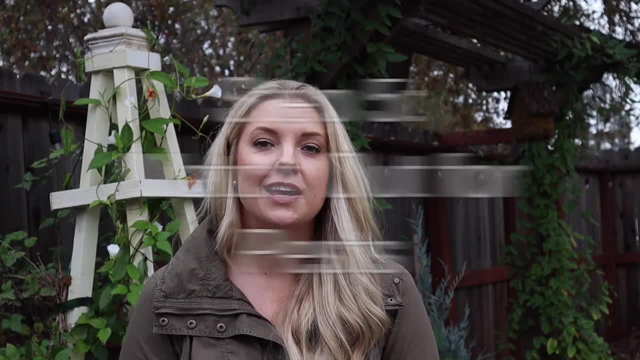 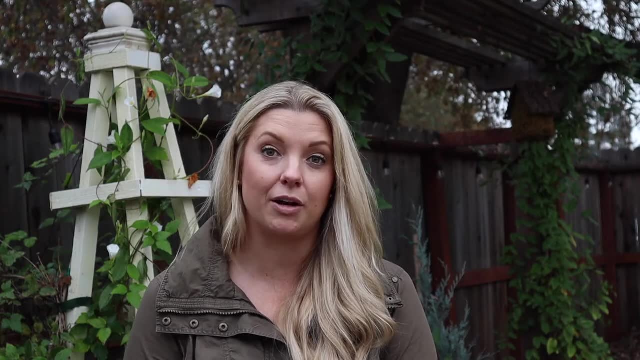 Okay. so step 5 in my gardening basics for beginners is to watch out for pests. Most gardens will deal with their fair share of pests, and that can ruin all your hard work very quickly. You will know you have pests by looking closely at your flowers or leaves. 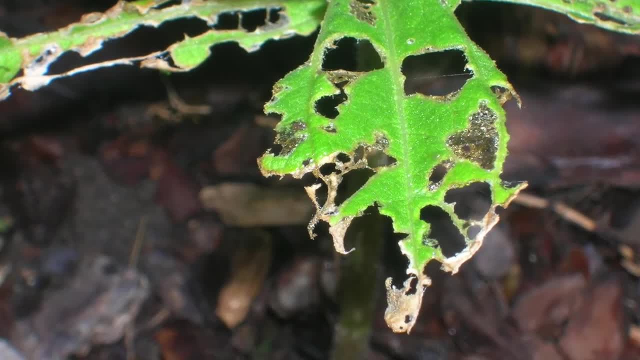 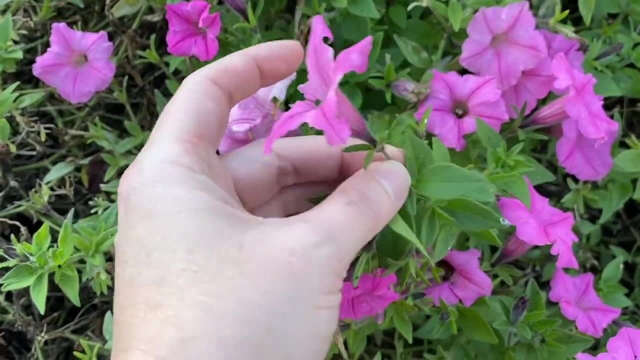 If they look chewed on, you most likely have something in the garden taking a little品. As a beginner, the easiest thing to do is to take a sample of a leaf to your local garden center to have them diagnose it for you. to your local garden center to have them diagnose it for you. they should be able to tell you what. 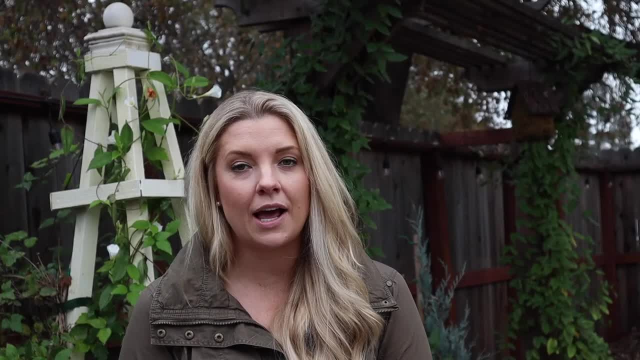 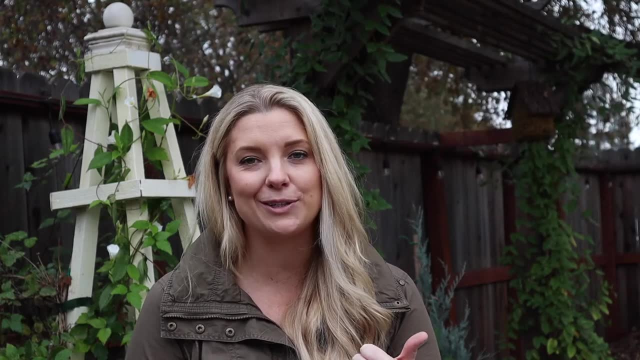 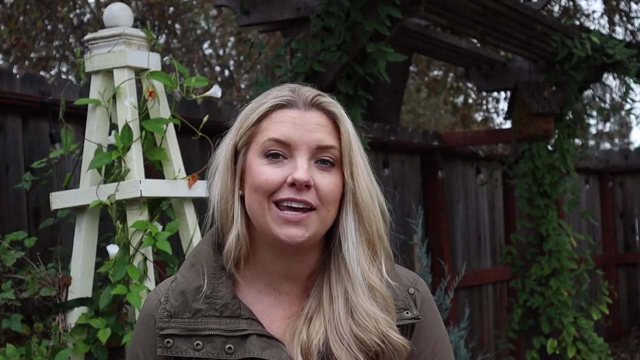 could be eating your plants and what you should do about it. here in northern california, the main pests i deal with are bud worms that will eat your entire flower off of your plant if they get to it. earwigs, snails, slugs, white flies, just to name a few. there are easy ways to take care of this. 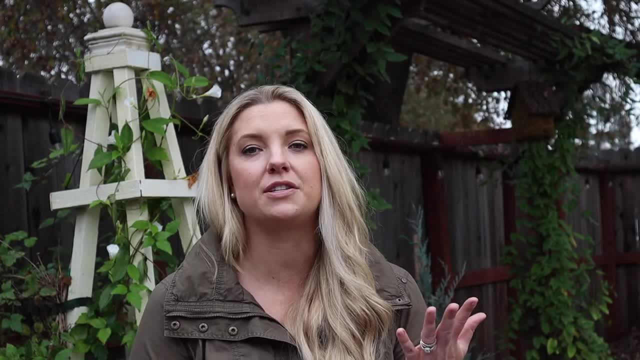 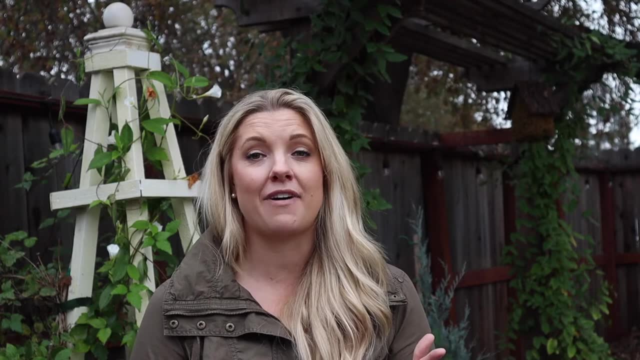 problem and manage these pests. you just have to know what you're dealing with to know what to do. step six: your plants are hungry, just like humans. we need water and food to survive. your plants need water and food to survive as well. each type of plant has a different 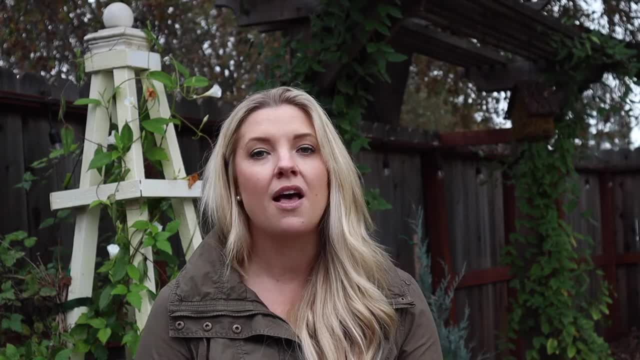 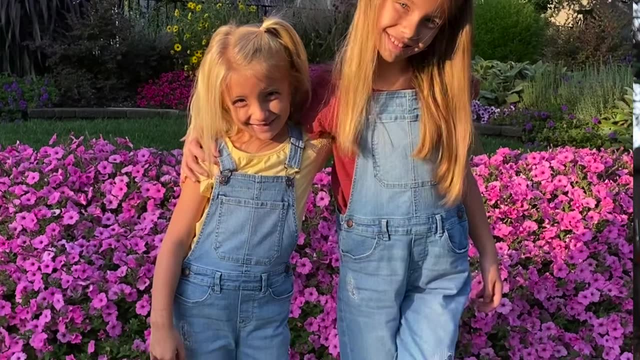 fertilizing requirement and a good rule of thumb to think about is: the more blooms, the more color the plant has, probably the more fertilizer it's going to need. take, for example, my supertunia vista bubble gums. they're probably the most abundantly colorful plant there is, and 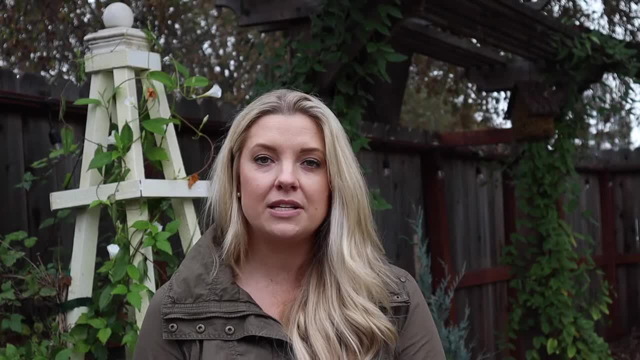 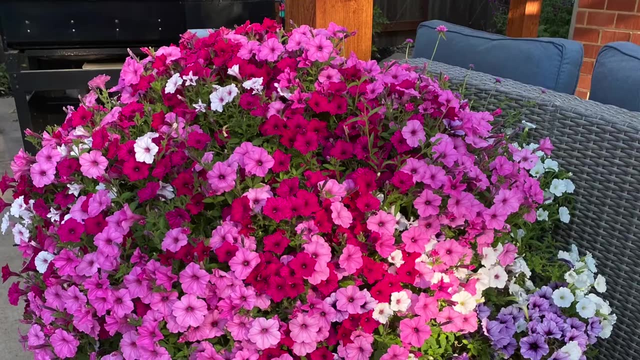 therefore, they need food every week during the growing season. compare this to a perennial that only blooms for a few months out of the season and they might only need a dose of fertilizer once or twice a year. i think that once i started actually feeding my plants, they became 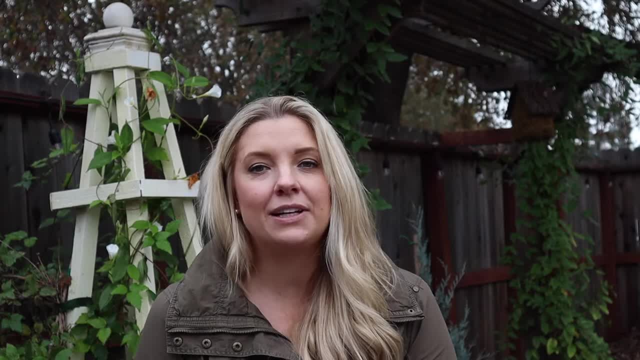 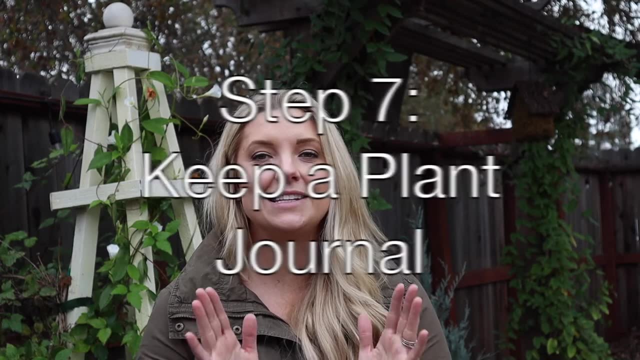 more vibrant and put on a show to thank me. i like to keep my fertilizing schedule set in the calendar on my phone so i have reminders to tell me when it's time to go feed my plants. step seven is keep a plant journal. this is a ton of information and there's no way anyone can 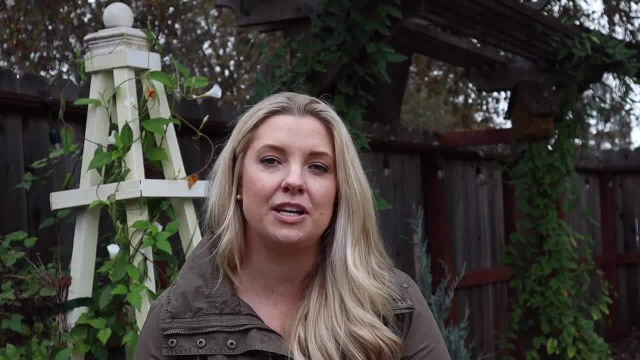 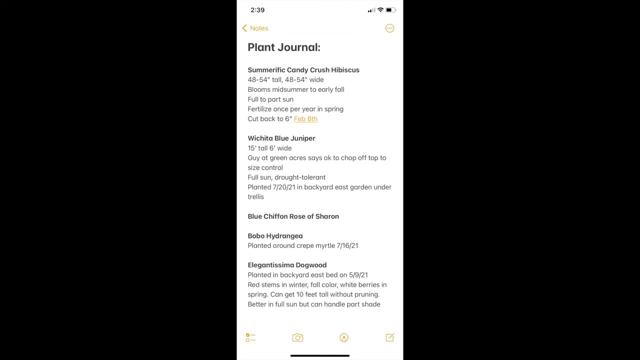 remember all of it. i like to keep my plant journal in my phone so i can look back on all the information that i have. i like to look on the plant tag and note when i can expect it to bloom, how much and when i should be fertilizing, and also when and how i should. 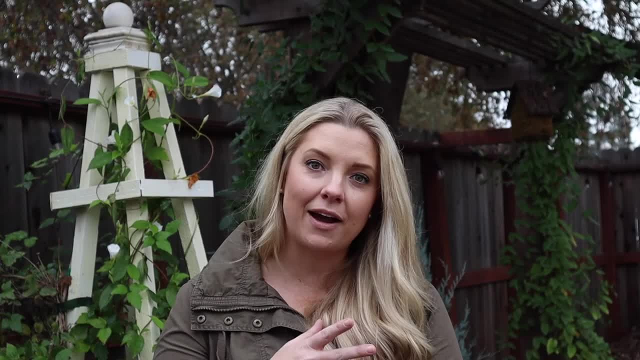 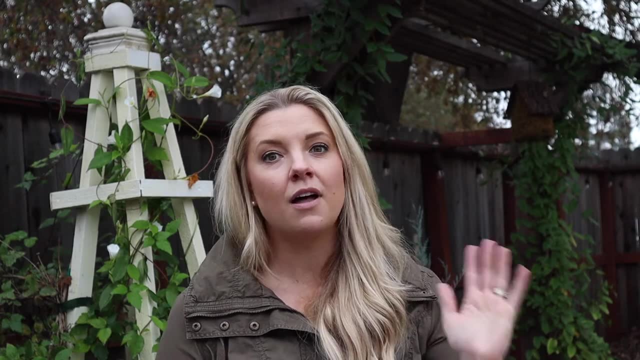 prune the plant if needed. having this allows me to look back on my notes from when i first bought the plant so i can remind myself what i need to do to treat the plant accordingly. so this has been a lot of information. i know i felt the same way when i started gardening: there was so much. 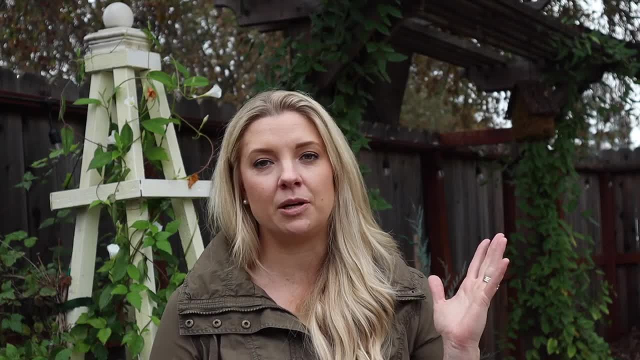 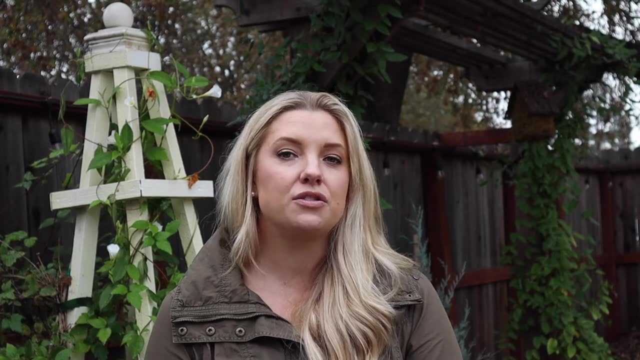 information to learn out there and i felt like i was never going to be able to grow anything. the true secret is, gardening is an art, it's not a science. it's trial and error, and humans have been gardening for hundreds of years and have done a great job at it. we didn't always have